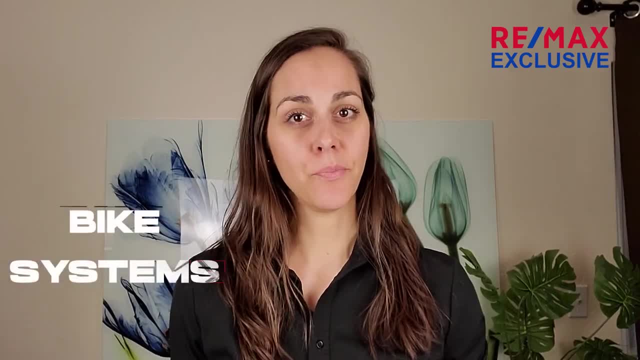 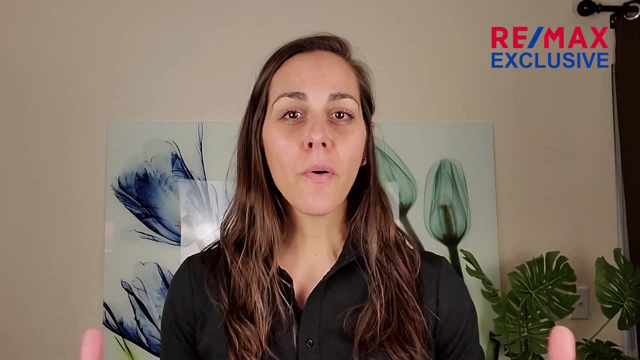 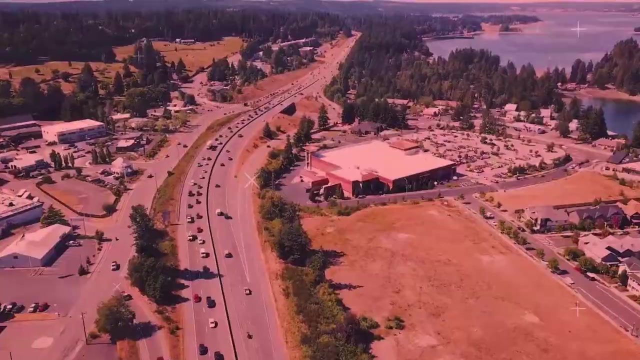 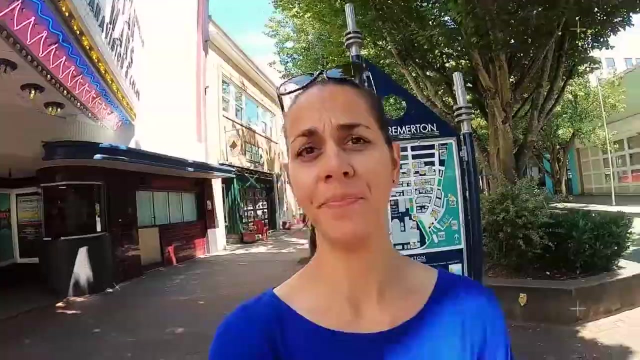 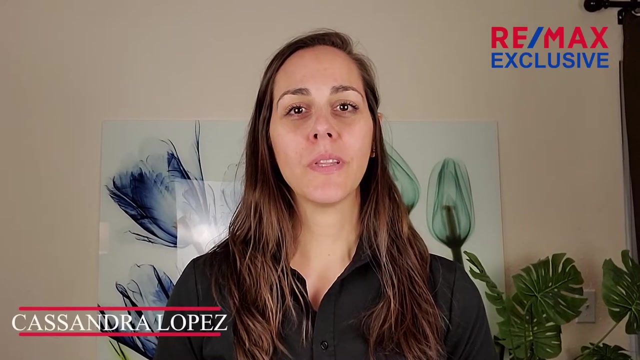 In this video we're talking all about our bike systems in Bremerton and Kitsap County, whether it's on-road, off-road, commuter, recreational. We're going to talk about all the ways to get around right now. What's up everybody? It's Cassandra Lopez with the Living in Bremerton channel, If you're new. 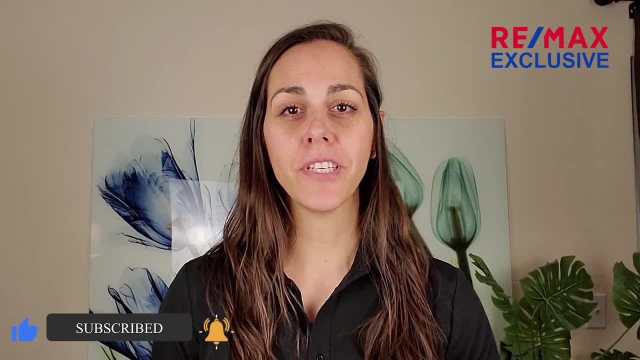 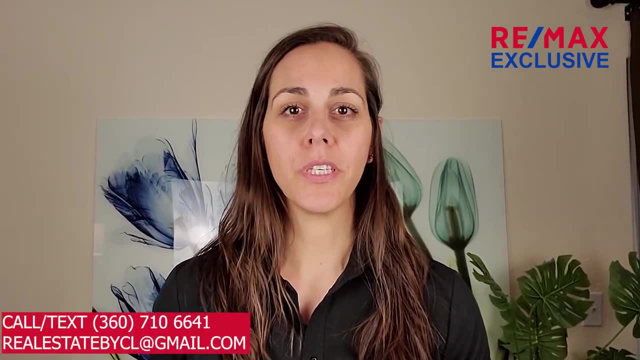 to the channel. go ahead and subscribe and tap that little bell so you're notified every time I upload a new video. If you're relocating to Bremerton, this is the place to be. This channel is all about living in Bremerton, So give me a call, shoot me a text, send me an email, let me 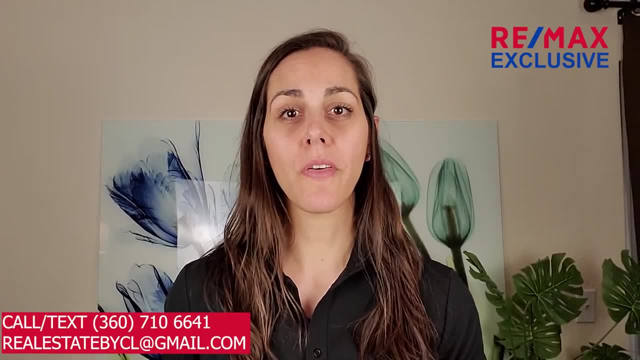 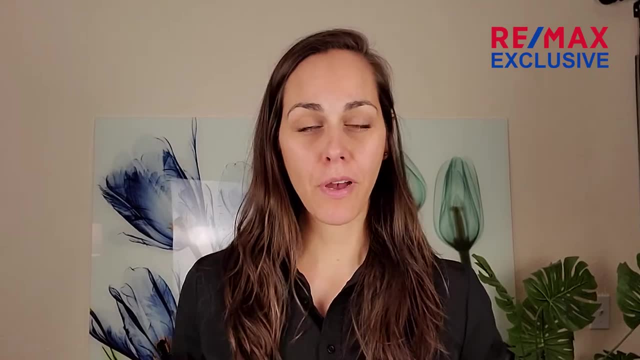 know how I can support your relocation to Bremerton and share this video with a friend who you think would benefit. So Bremerton, and the Pacific Northwest in general, is known for its plethora of outdoor resorts and resorts, So if you're looking for a place to live in Bremerton, you'll want to go to the city of Bremerton. There's a lot of outdoor activities year-round, biking included. A lot of people decided to hop on a bike for more exercise, or maybe to save money on their commute to work, or maybe to reduce their carbon footprint, or maybe a combination of the. 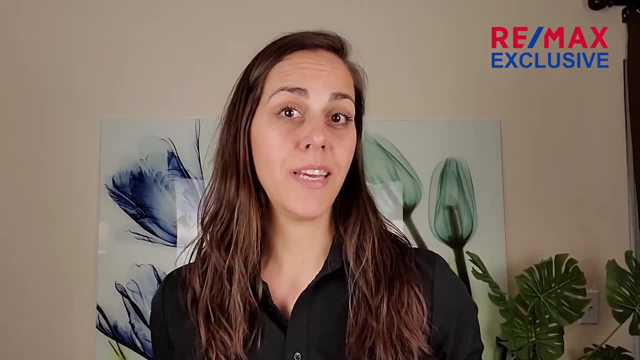 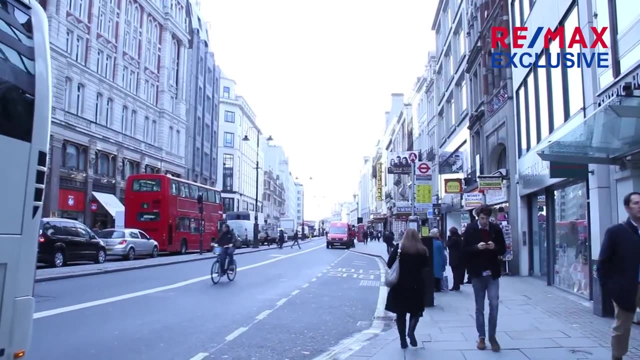 aforementioned. So it might surprise you to learn that the city of Bremerton, and Kitsap County in general, doesn't have a lot of bike-friendly roads, and by that I mean there aren't a lot of designated bike lanes. Right now, bicycle commuters share the road with vehicles. The city of Bremerton is known for its outdoor activities, Year-round biking included. A lot of people decided to hop on a bike for more exercise, or maybe to save money on their commute to work, or maybe a combination of the aforementioned. So if you're looking for a place to live in Bremerton, and Kitsap County both have long-term plans to add more designated bike lanes to our roadways, but all of that is super dependent on a myriad of factors, such as the current road width and if they are even capable of expanding the road to add a bike lane. 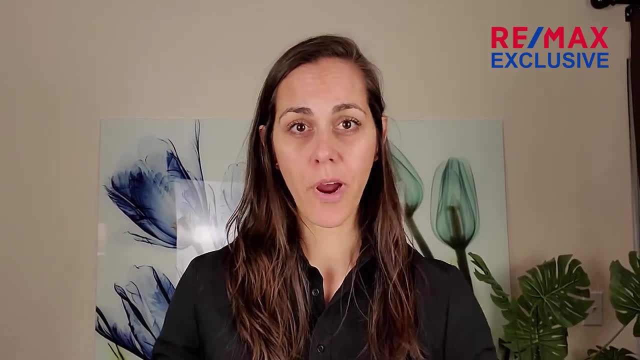 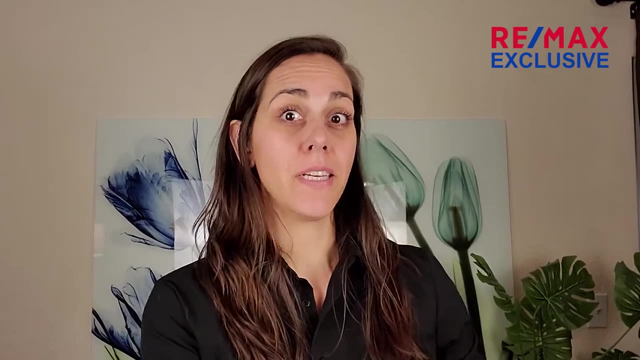 A lot of times the property owners of the private property will kind of come into the street, maybe at least to the sidewalk a little bit, and so they would have to like sacrifice like three feet of the property owner's property on either side, and so property owners vote that down, and of course, 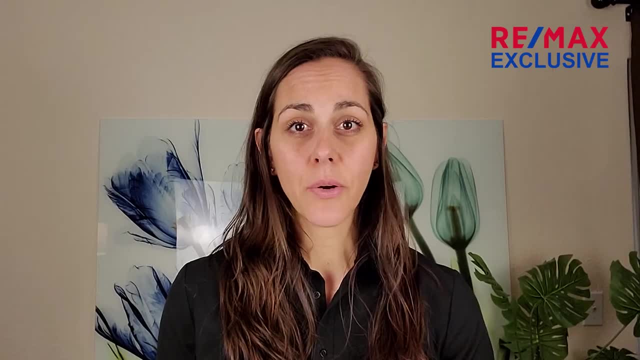 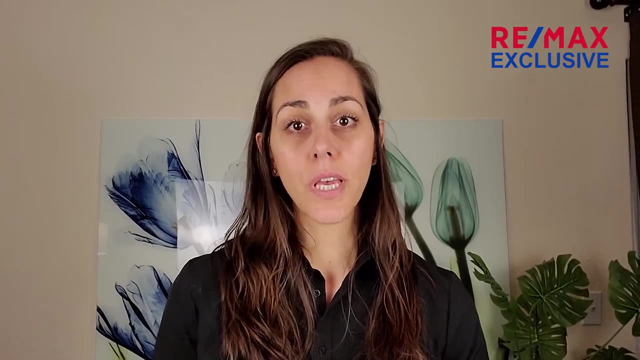 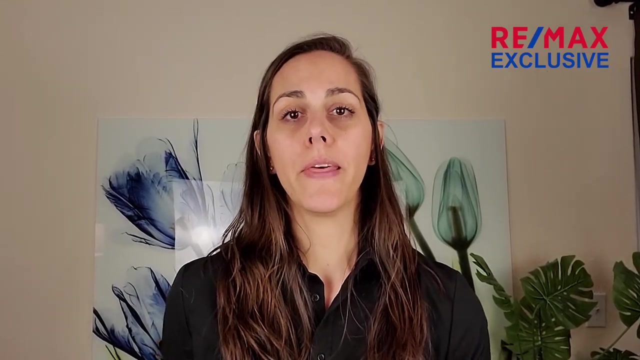 that's not going to happen. Also, around here we have a ton of waterways, like whether it's shoreline or creeks or rivers or streams, and a lot of those carry special setback requirements and so if you get any closer to those, you know you won't be able to improve upon that property or that land. adding a wider road or more bikeways. A lot of municipalities are waiting for the development of land, so you know projects coming down the road, like a housing development or or what. have you any kind of improvement? in which case they'll add a bike lane. at that point when. everything's already torn apart and under construction. anyway, when they put it back together, they'll just add a bike line. but you know all of those projects, they're staggered and they're slated, and maybe a lot of them don't have timelines yet, and so there's really no way to know. when these bike lanes will become available, if ever. I've provided links for the city of Bremerton, county planning departments, the plans for the improvements on the bike lanes in the description below. Now, if you're biking for recreation and you just want to take a day to bike around town, 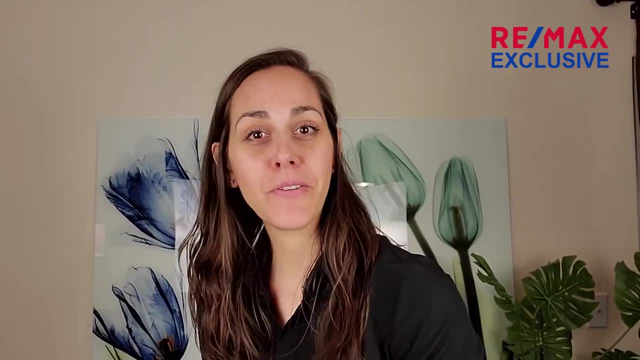 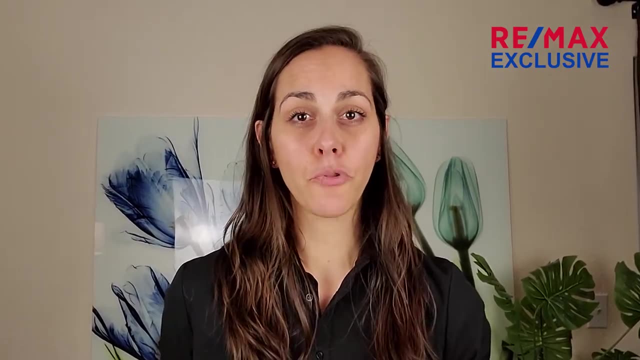 or bike around the county or the shoreline or up to a different county or out to an island. there are tons of designated routes that you can take that are already pre-planned and mapped out for you. A lot of them are on roads, so you're going to be sharing the roadway with vehicles. 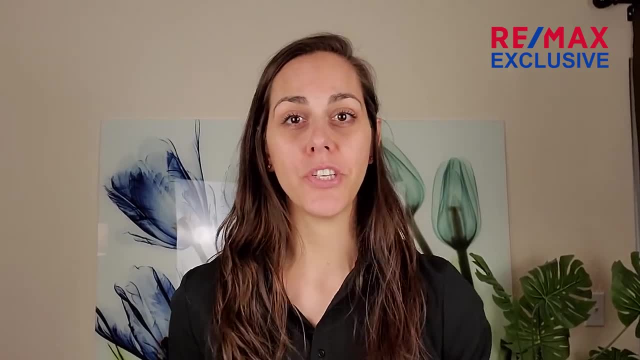 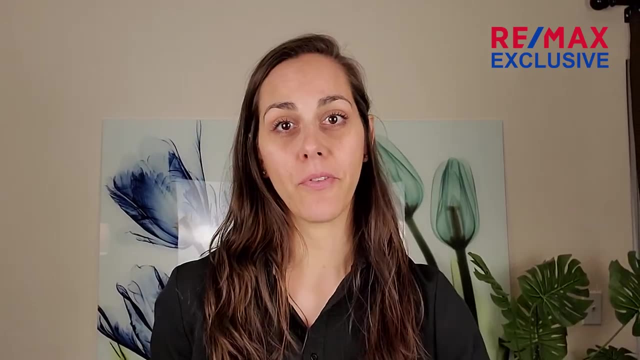 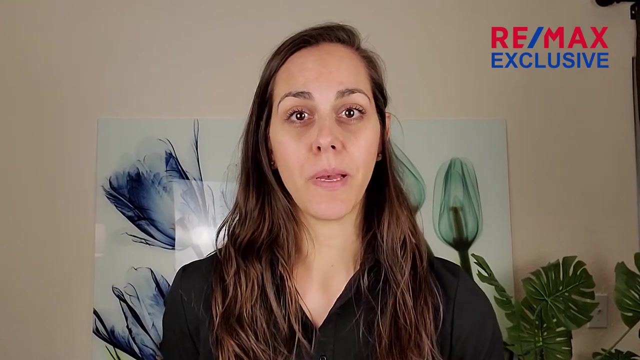 and they transition to off-roads, And so you have kind of a combination of both. I've provided in the description a link to a site where you can access all of the bike routes. so if you're planning ahead or planning a trip or want to take advantage of that opportunity, this is a great resource for you to be able to do that. 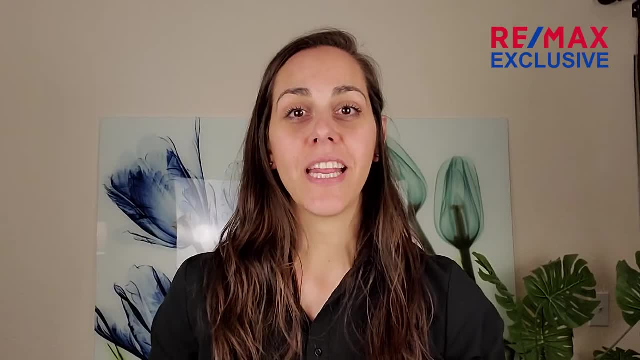 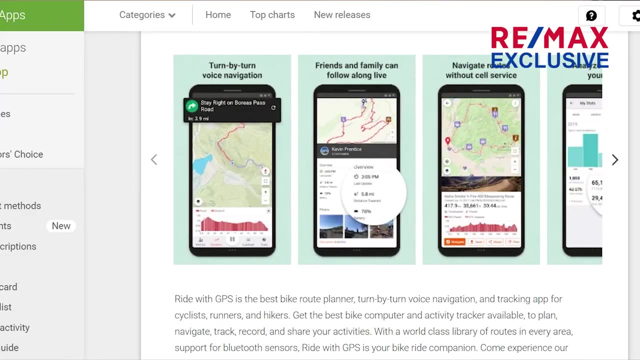 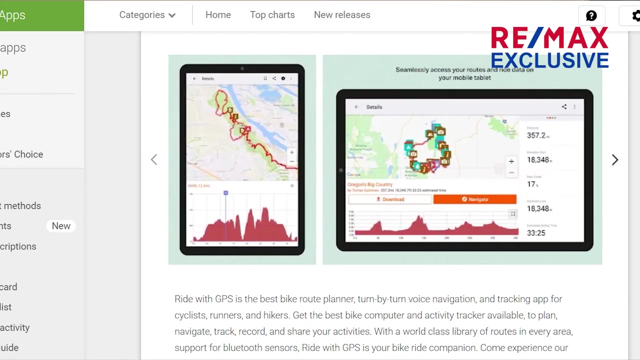 And, as always, there's probably an app for that. there's an app called Ride with GPS and basically you can access any bike route anywhere in the country and you can filter by distance, location, elevation, climb, on-road, off-road, a combination all these factors, so you can plan your trip well in. 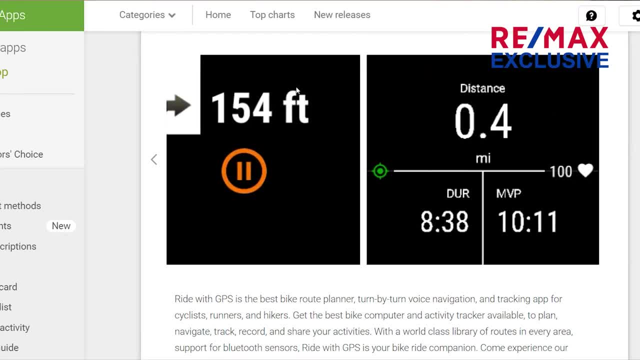 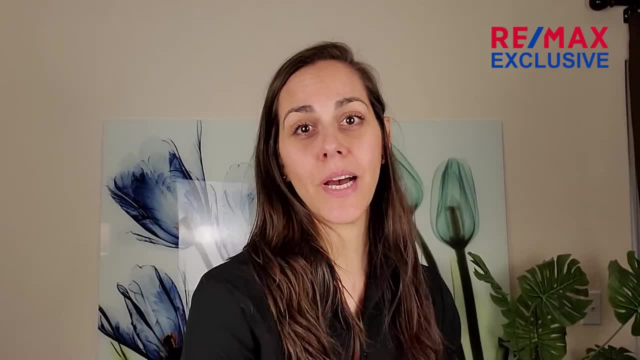 advance and know what kind of gear you need to bring, know what kind of safety stuff or snacks or water, anything how long you're going to be. A lot of them have multiple ferry rides: if you're taking a ferry out to an island, riding around the island and then back to the mainland. so you want to plan. 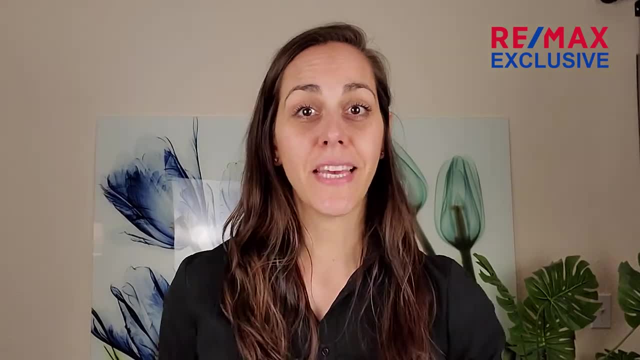 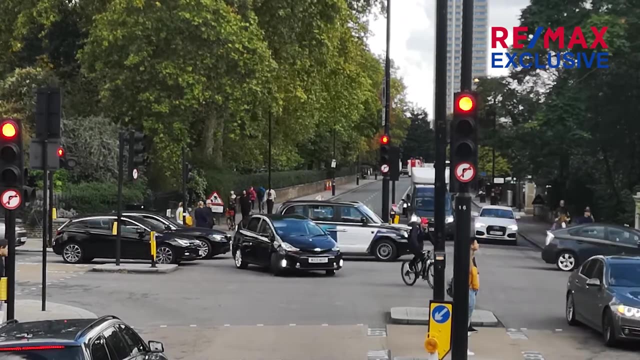 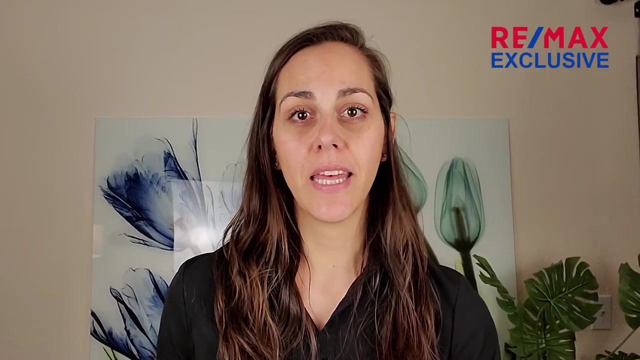 for that. So a lot of cool stuff going on there for you to take advantage of, And that's a good segue into my next point, which is, if you're going to share the roadway with other vehicles, it's important to know which areas have road closures or road construction or delays, and so I've provided. 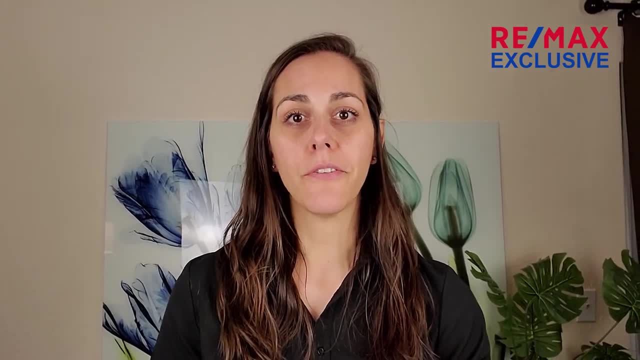 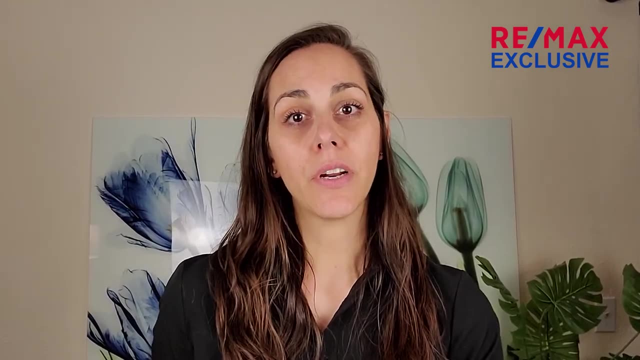 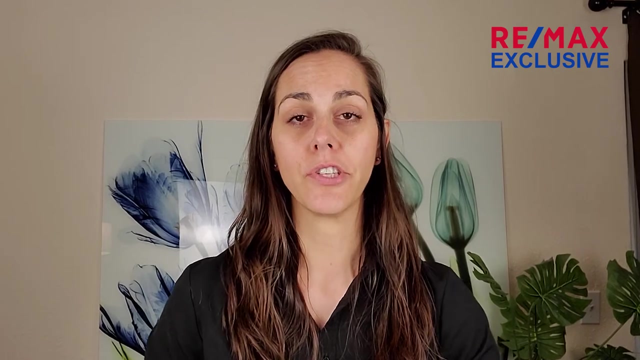 a link in the description for a county site which offers current projects going on, so road closures and delays and detours. In addition, they also send out emergency information, so if there's a tree down blocking a roadway, or maybe a vehicle accident blocking a roadway where they have to shut the. 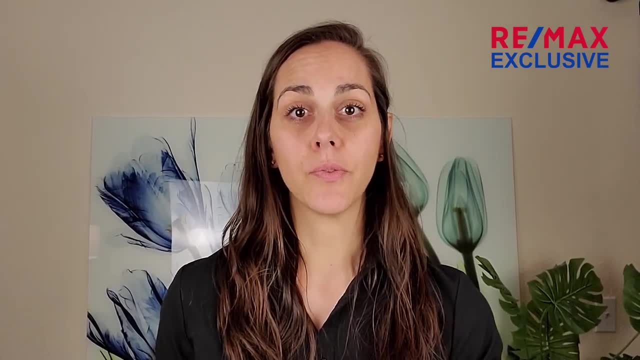 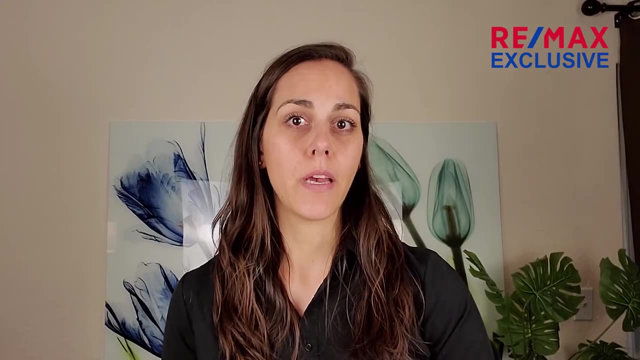 road down. they will provide real-time information on that as well. You can actually check that out and sign up for periodic alerts. I get an email, I think once every Friday, which shows me these are the roads that are going to be closed for the weekend, and although I don't ride my bike on the 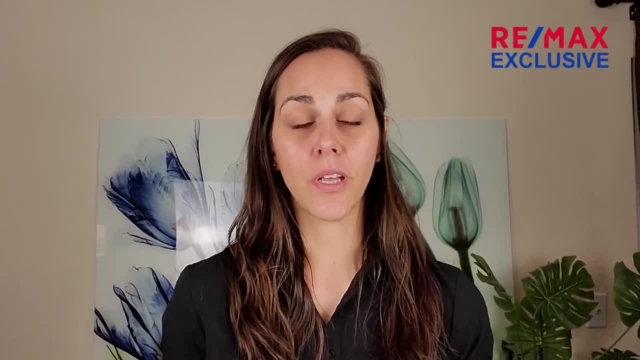 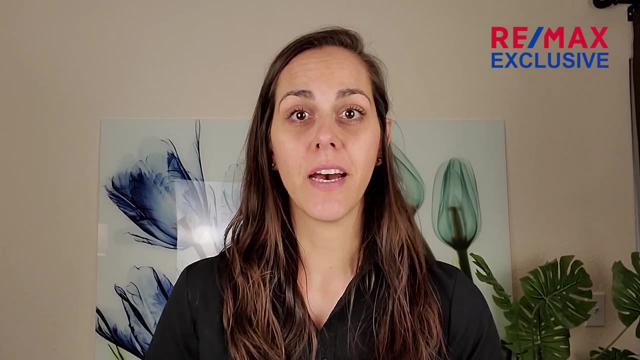 roadways. very often. it's helpful if you're just driving in a car too, because I do a lot of showings on the weekends and so it's helpful for me to know if I need to do a detour or plan my ride out accordingly. So I've provided the link in the description for that super helpful resource.